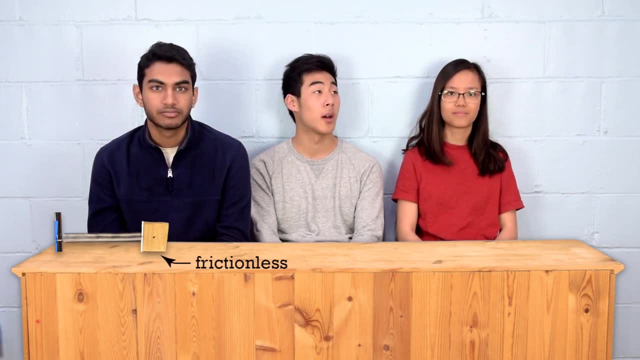 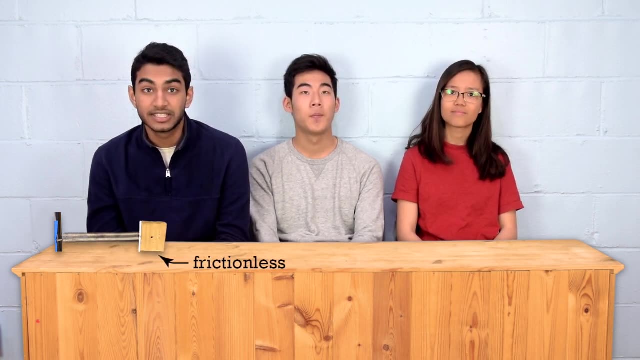 how did you demonstrate it Right? I mean, the mass is not slowed down at all. Yeah, the amplitude of your demo is constant the whole time, which does not make sense. There has to be at least a little bit of friction that slows it down. 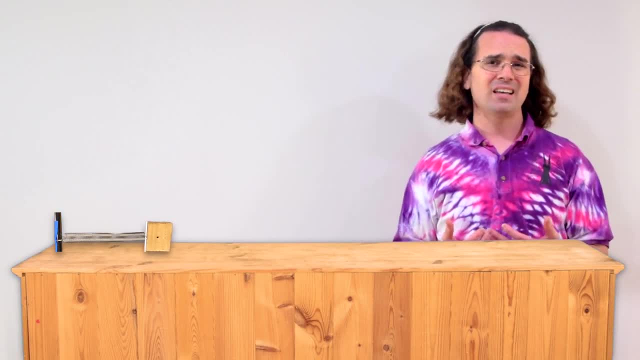 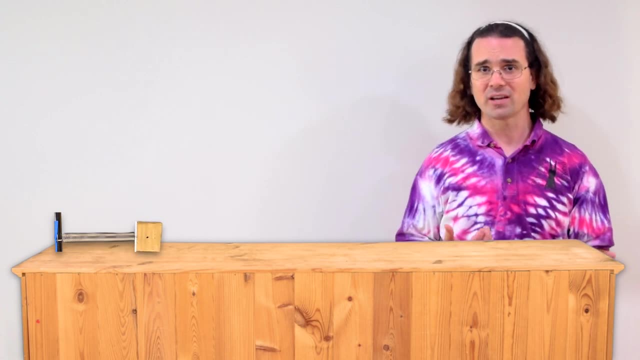 and slowly decreases the amplitude. Well, first off, realize I looped the video. You were just watching the same single cycle of the mass spring system over and over again. Second, it is actually not a horizontal mass spring system, It is a vertical mass spring. 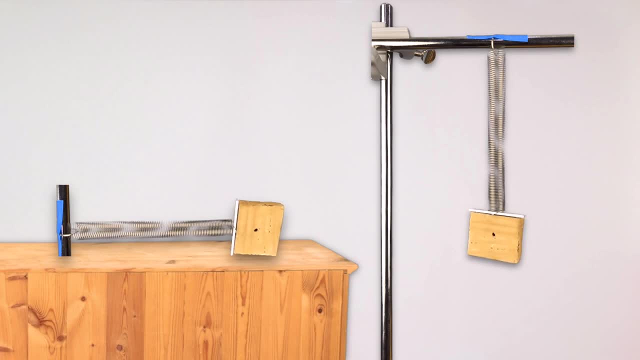 system that I rotated 90 degrees. Dude, that's totally cheating. Actually, it is not cheating, because horizontal and vertical mass spring systems both behave in the same way. They both behave in the same way. The difference is that when a mass spring system is vertically oriented, 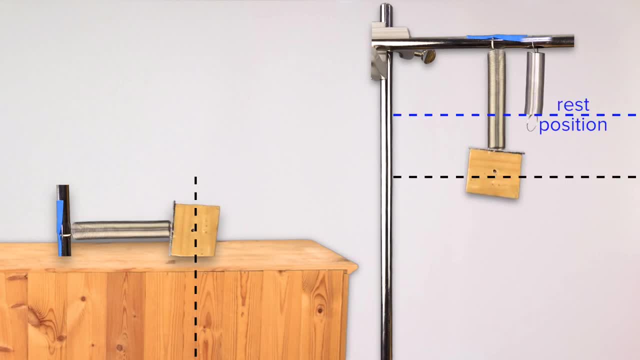 the mass oscillates around a location which is lower than the original equilibrium position. I'm not going to go through a strict derivation of how it works. However, realize it oscillates around where the mass spring system is at rest, with the mass hanging on it. At this point, the net force in the y-direction equals zero. 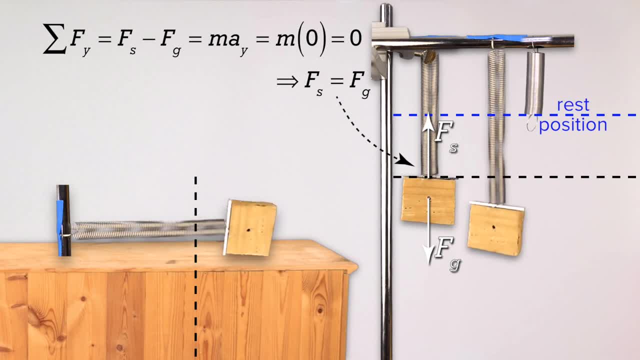 because the upward spring force and the downward force of gravity cancel one another out. Therefore, in a vertical mass spring system, the net force in the y-direction, which is the restoring force causing the mass to be in simple, harmonic motion, includes both the upward spring force and the 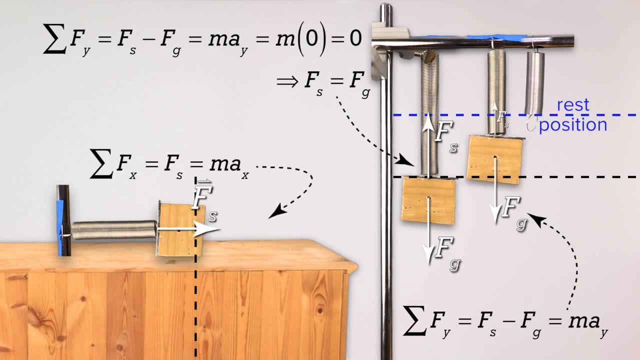 downward force of gravity. In a horizontal mass spring system the only force acting in the x-direction is the horizontal spring force, So that equals the net force in the x-direction, which is the restoring force. that causes simple harmonic motion. Both the horizontal and vertical mass spring systems oscillate from position one to the other. 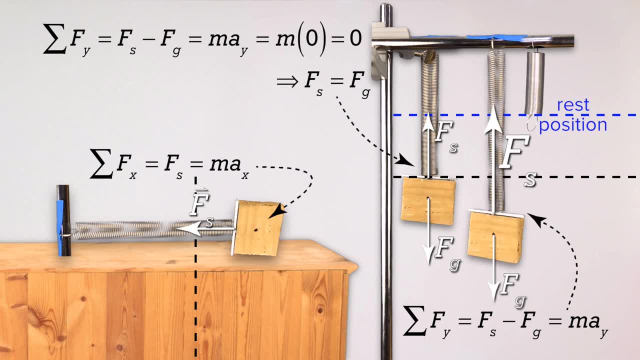 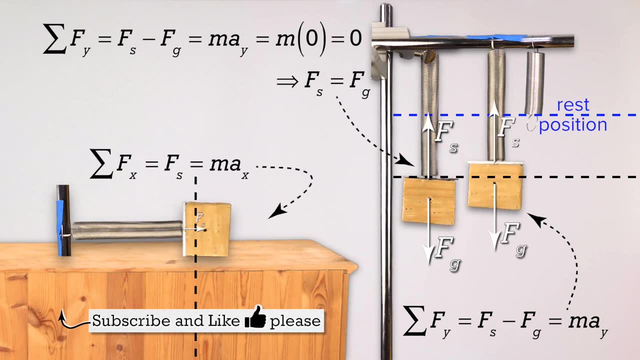 to 2, to 3, to 2, to 1, to 2, to 3, to 2, to 1, and on and on, because they are in simple harmonic motion. Sure Thanks, Mrp. I guess I should also point out that I did slow the video of the mass spring system. 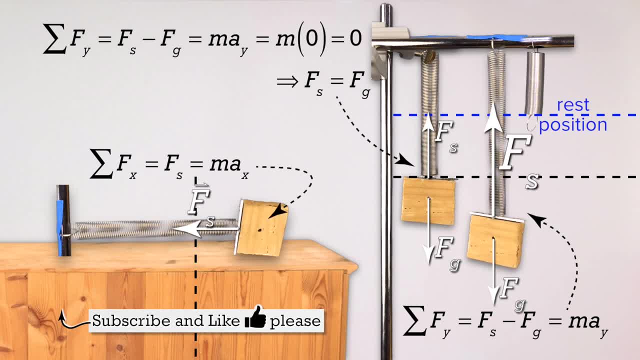 down to 1 eighth its normal speed. When I show the video at normal speed, it becomes much more difficult to understand what is happening. Thanks for doing that. Thank you very much for learning with me today. I enjoyed learning with you.